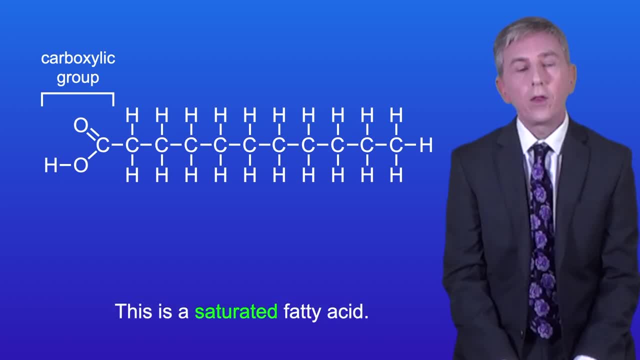 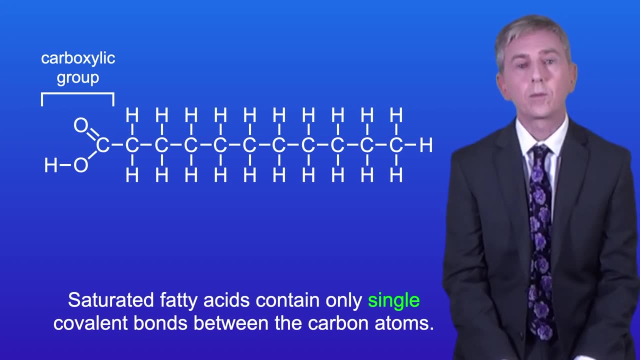 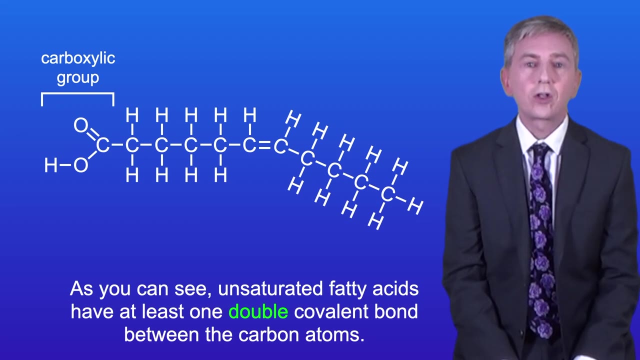 of carbon atoms bonded to hydrogen. Now this is a saturated fatty acid. Saturated fatty acids contain only single covalent bonds between the carbon atoms, and we can see those here. I'm showing you here an unsaturated fatty acid. As you can see, unsaturated fatty acids have at least 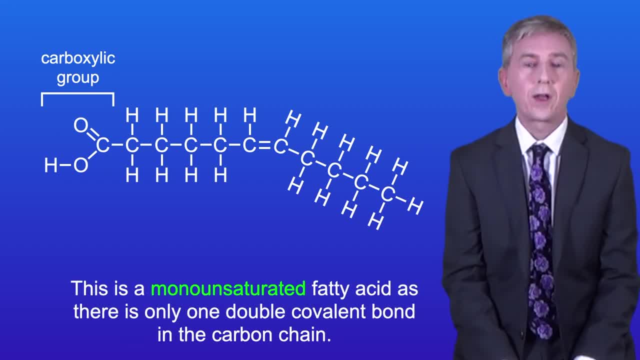 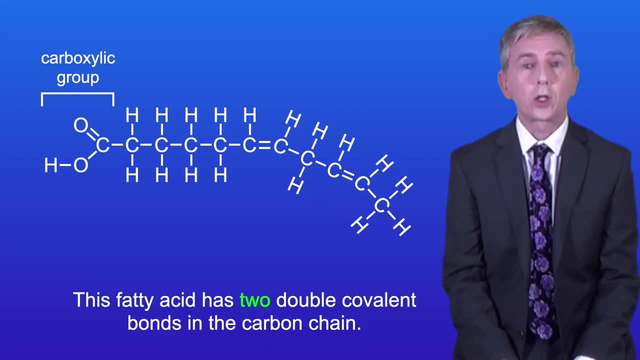 one covalent bond between the carbon atoms. This is a monounsaturated fatty acid, as there's only one double covalent bond in the carbon chain. This fatty acid has two double covalent bonds in the carbon chain, So this fatty acid is polyunsaturated. Coming up, we're going to look. 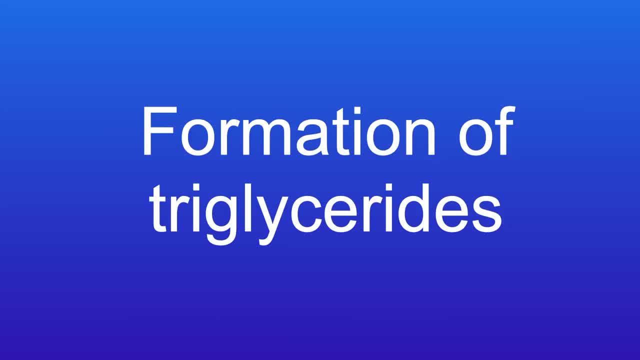 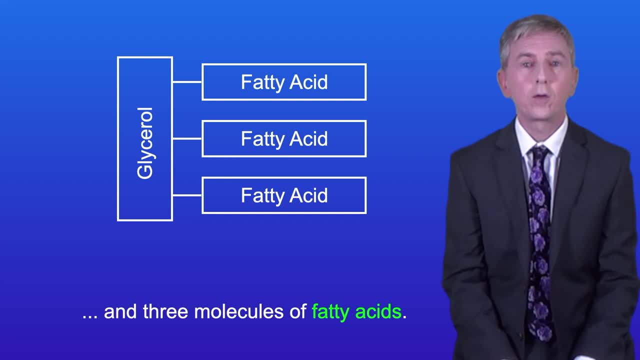 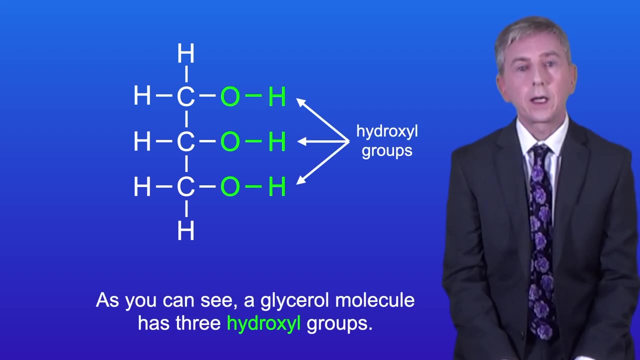 at the formation of triglycerides. Okay now, as we saw before, triglycerides are formed from one to three hydroxyl groups. I'm showing you a molecule of glycerol here, and I would recommend that you learn this structure. As you can see, a glycerol molecule has three hydroxyl groups. 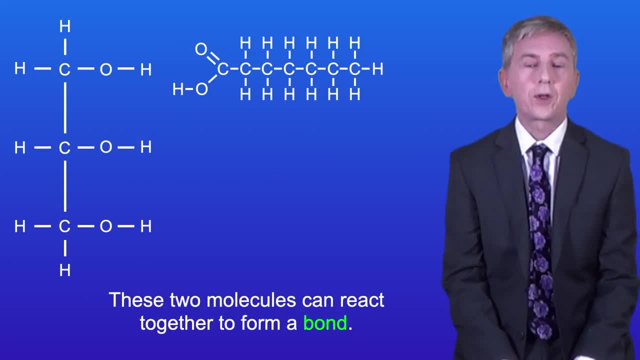 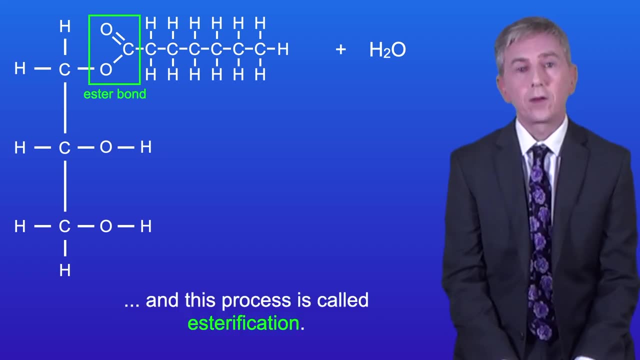 Here's a glycerol molecule and a molecule of fatty acid. Now these two molecules can react together to form a bond, and I'm showing you that here. This is called an ester bond and this process is called esterification. In this reaction we also make a molecule of water. So this is an example of a. 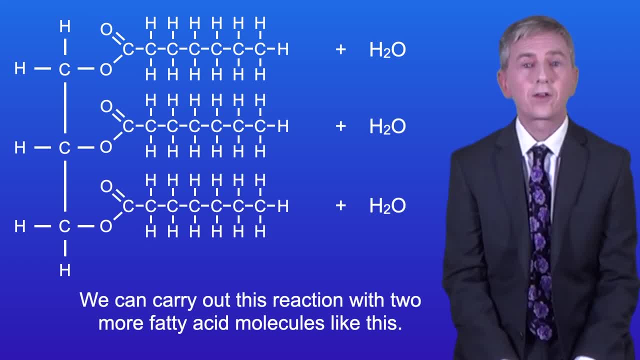 condensation reaction. We can carry out this reaction with two more fatty acid molecules like this, and this is the structure of a triglyceride molecule. Now, as we said before, fats and oils are a major source of energy in the human diet. 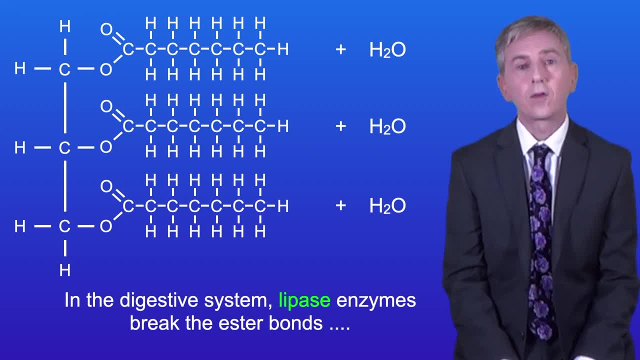 In the digestive system, lipase enzymes break the ester bonds, releasing the glycerol and fatty acid molecules. This reaction requires three water molecules and is an example of a hydrolysis reaction. Now there are a couple of final points about triglycerides that you need to understand. 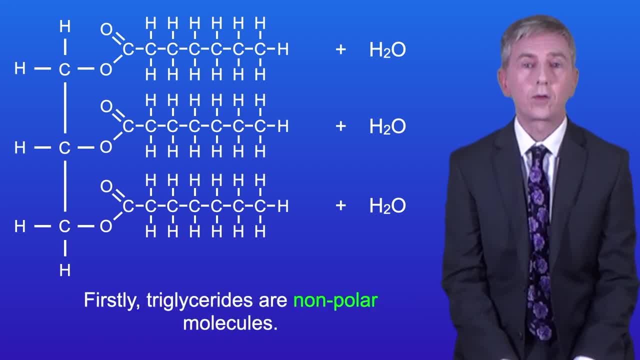 Firstly, triglycerides are non-polar molecules. This means that they're hydrophobic, In other words, they do not dissolve in water. This explains why triglycerides are used as waterproofing, for example, in aquatic birds. Secondly, because triglycerides contain a large number of carbon. 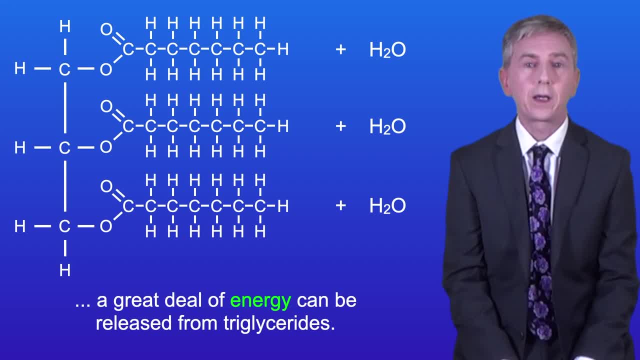 and hydrogen atoms. a great deal of energy can be released from triglycerides and we'll see that in more detail in the topic on respiration. In the next video we look at the category of lipids called phospholipids. Subtitles by the Amaraorg community.